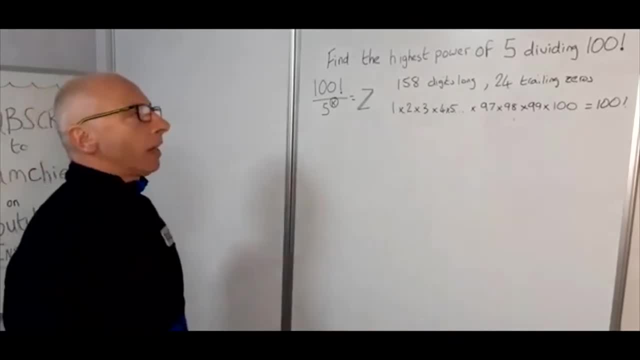 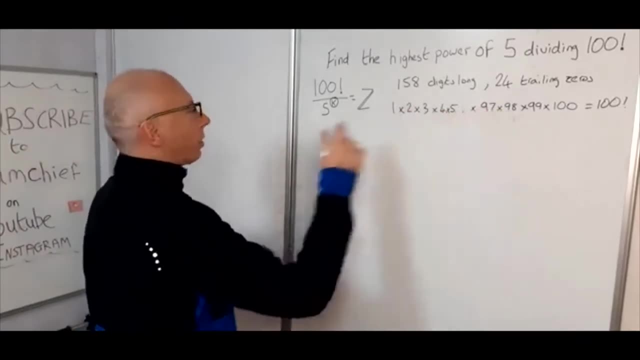 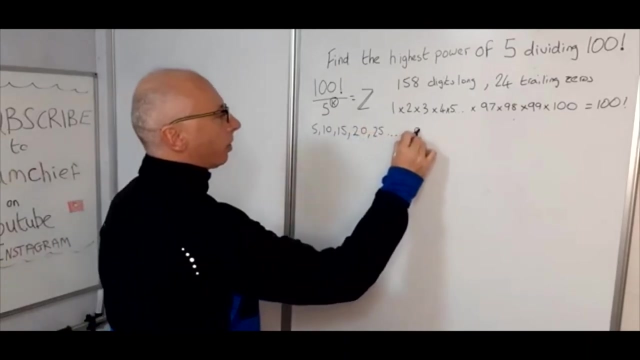 us find a number that divides by 5.. So what we can say is we find all the multiples of 5 that give us into the 100.. So we've got 5, 10, 15,, 20, 25 and so on all the way up to 95 and 100. 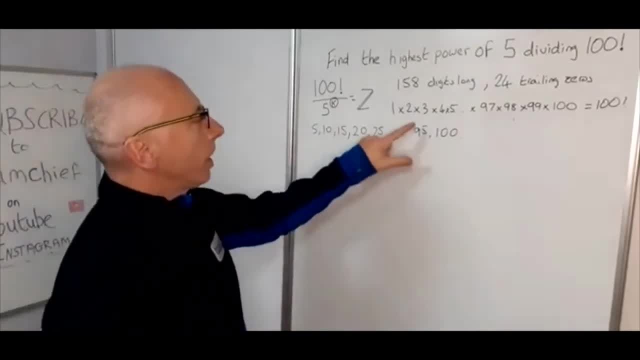 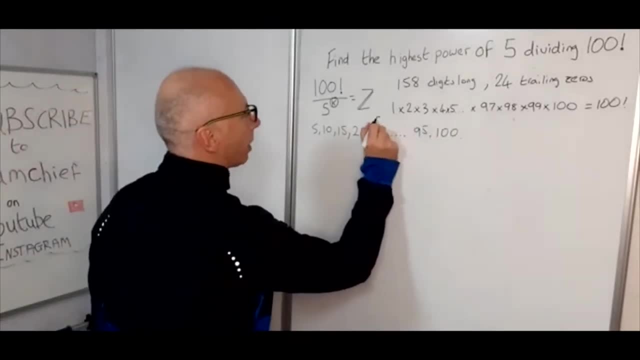 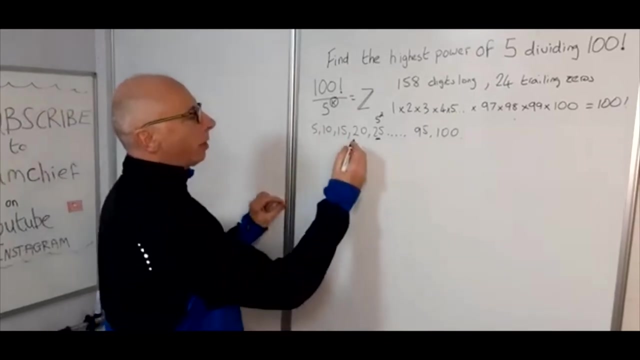 So what we're interested in here is all of these here, within this product here. Now interesting to see here is 25 is 5 squared, whereas these ones here their prime factorization, this one would be 5 to the power of 1 times 2 squared. This one here. 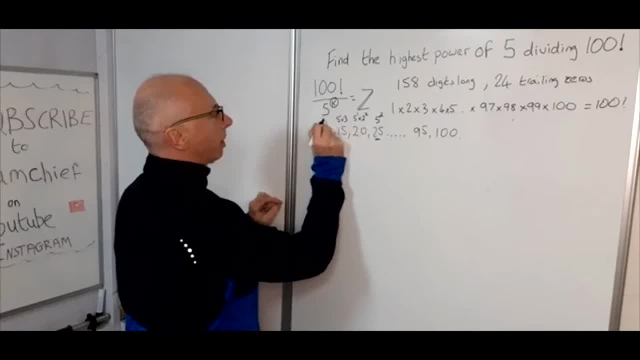 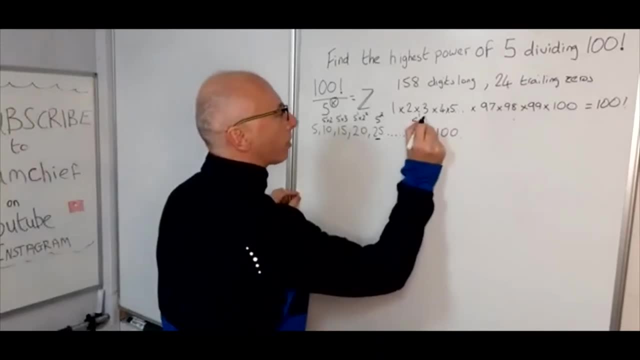 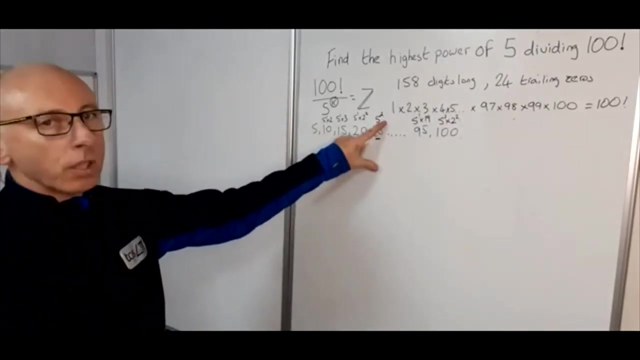 is 5 to the 1 times 3, and this is 5 to the 1 times 2, and so on. This one here would be 5 to the power of 1. 1 times 19, and this will be 5 squared times 2 squared. so we've got some fives that appear twice. 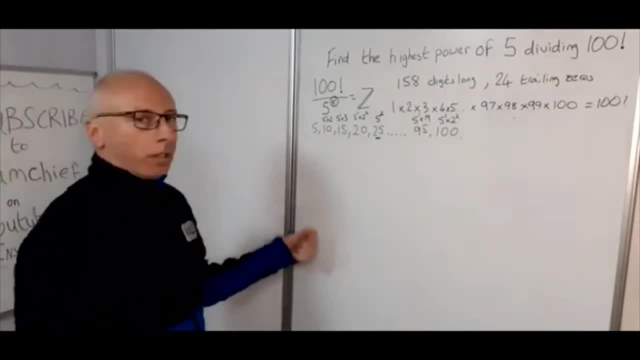 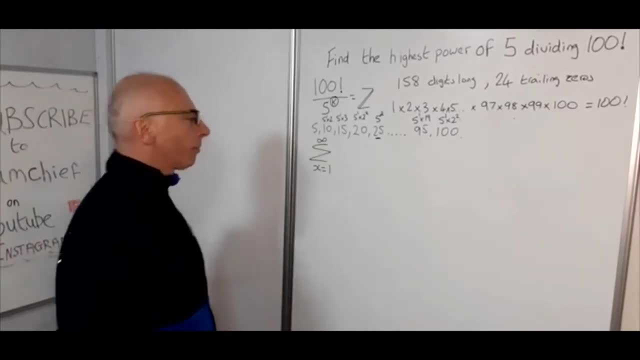 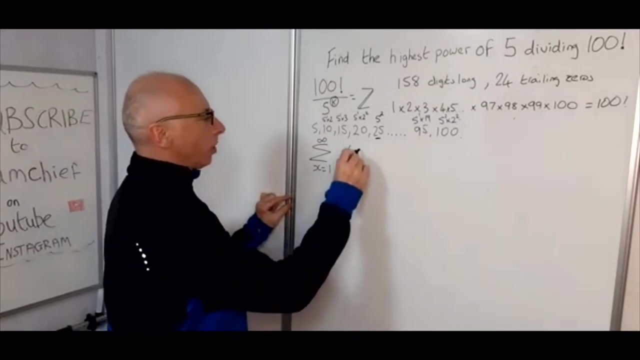 and some fives that only appear once. so we need a summation formula. so what we can say is we go from x equals 1 to infinity, and then the number we're interested in is the number that's used for the factorial. so we'll just call that the number n, and then we'll divide that by the prime number. 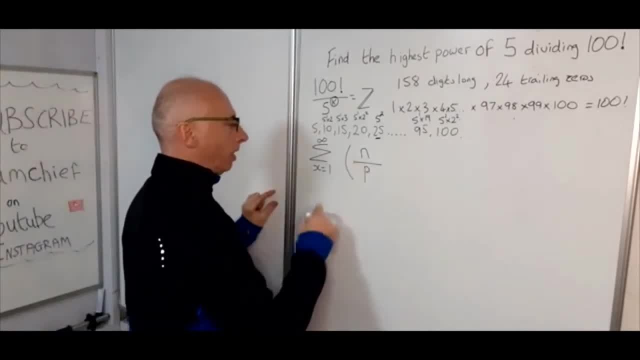 which is in the denominator. we'll just call that p and it'll be p to the power of x, and that will be sorry. it will be a normal bracket. it will be a floor function, because what we're interested in is only integers, so we need a floor function to. 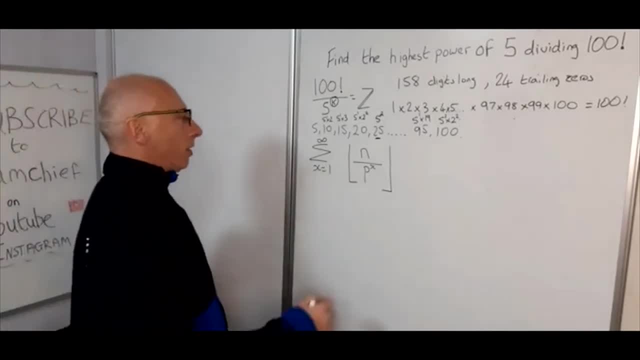 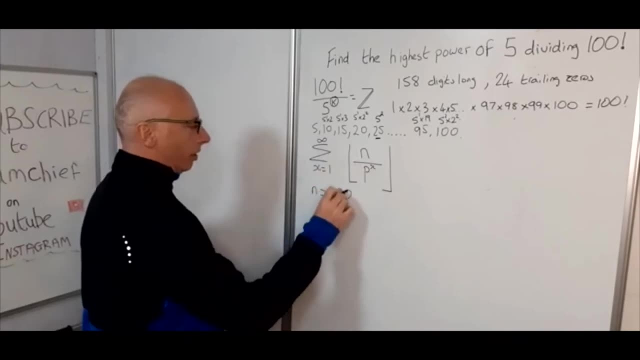 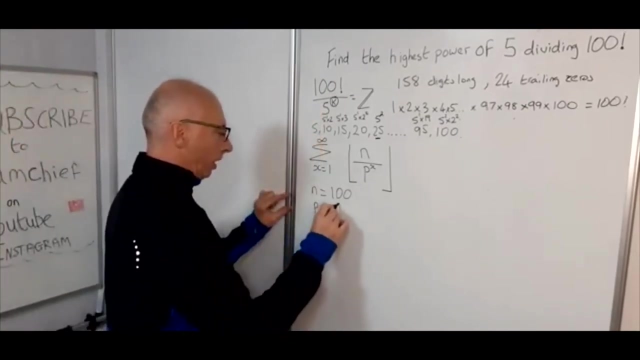 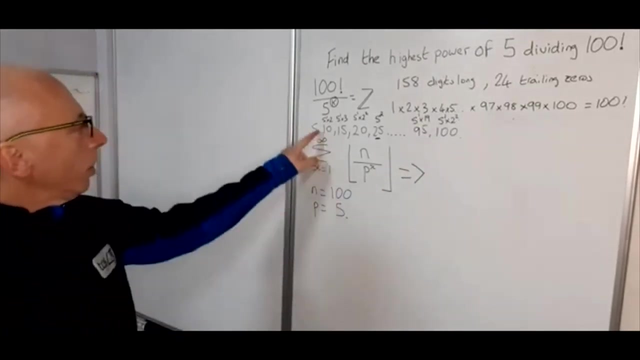 break this down as an integer. so what we now know we can say is: n is 100. so that's the factorial number we're interested in, and the prime number we're interested in is five. so p equals five, okay. so, looking at this number here, our 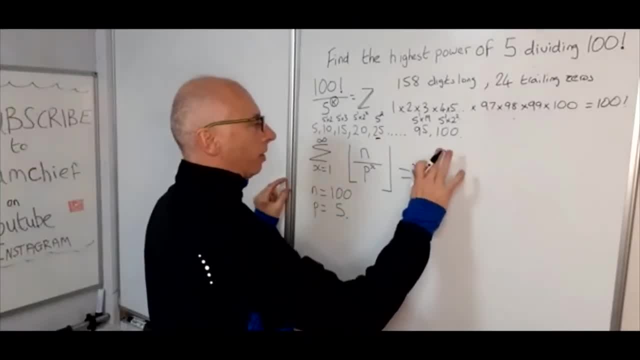 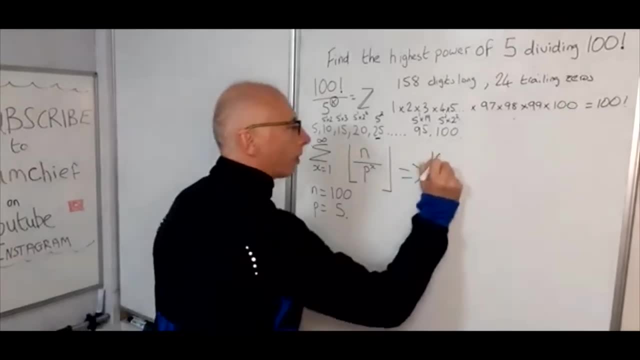 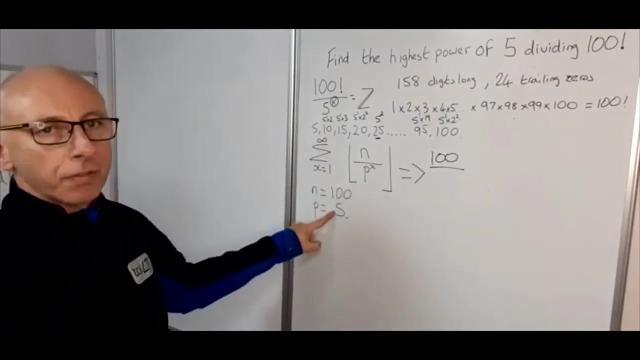 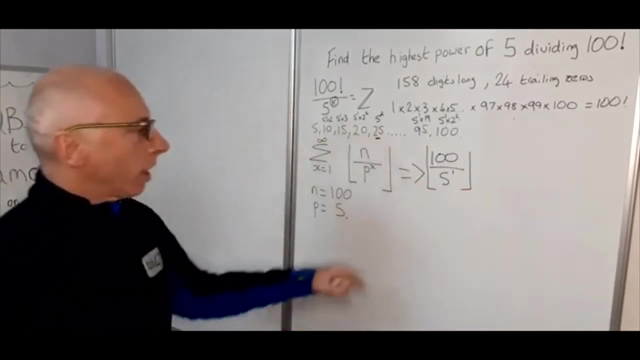 first one is n, so we just change it into: sorry, that's 100, so our n is 100, so i type in 100 and then we divide that by p to the power of one. that's the first one in here- and p is five, so five to the power of one, and that's a floor function. so 100 divided by five. 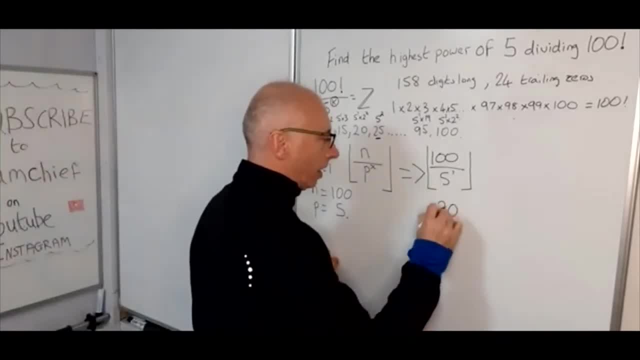 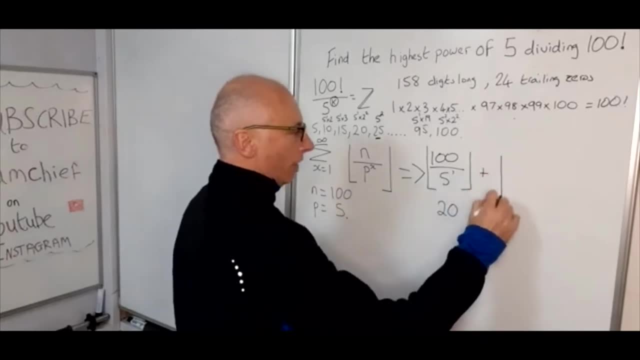 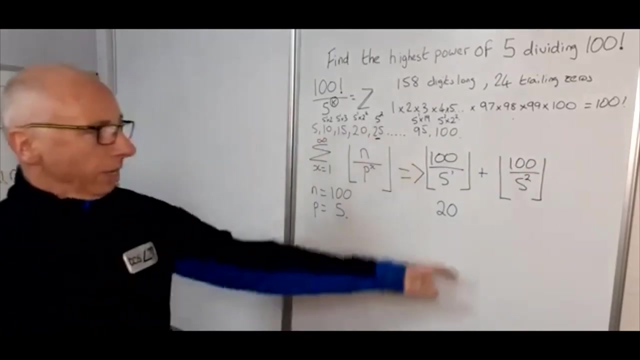 to the power of one. i'll just write that down here. that is 20.. 520 is 100. pretty straightforward, as it's a summation formula, our next one, enclosed in the floor function, will be 100 divided by 5 squared. now, 5 squared, we know, is 25. 100 divided by 25 is 4.. 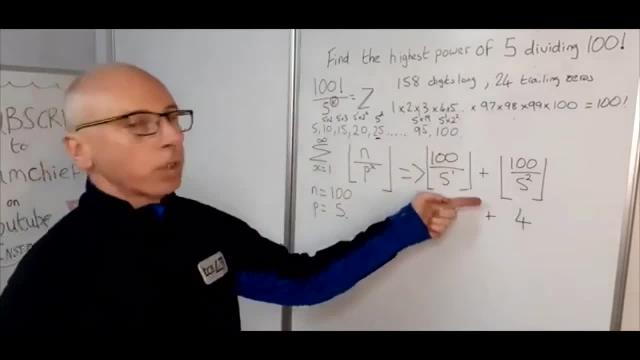 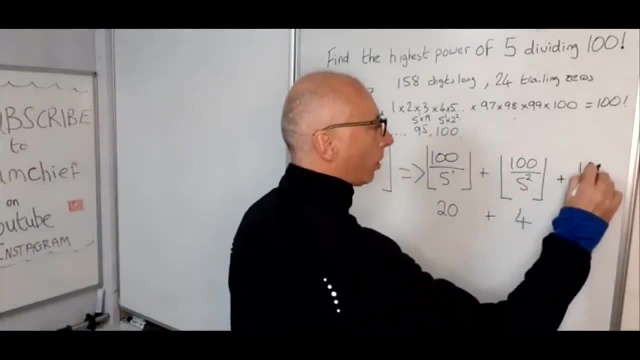 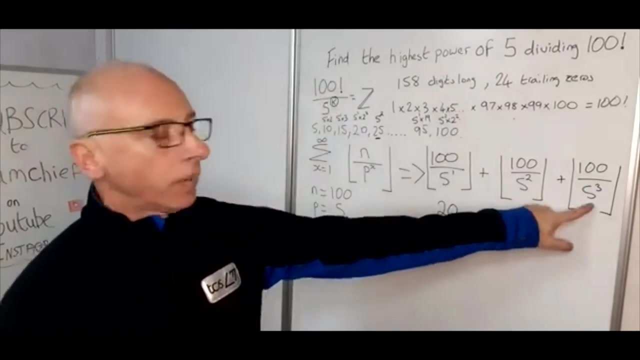 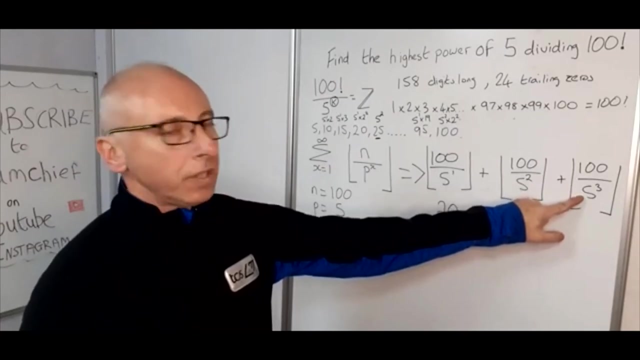 so our floor function here at the moment is not not looks like it's not needed. but when we come to the next one x equals three. so plus 100 divided by five cubed, we'll see here five cubed is 125.. so 100 divided by 125 is four-fifths. but four-fifths is less than one. so in the floor, 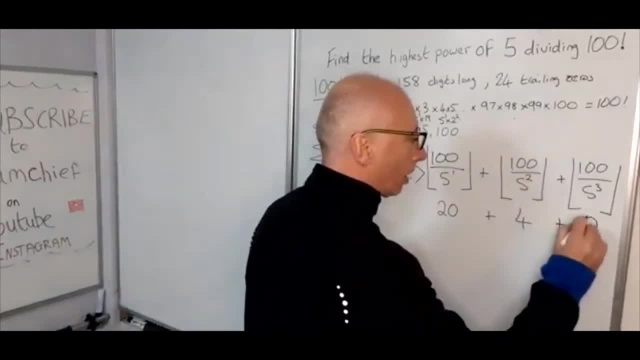 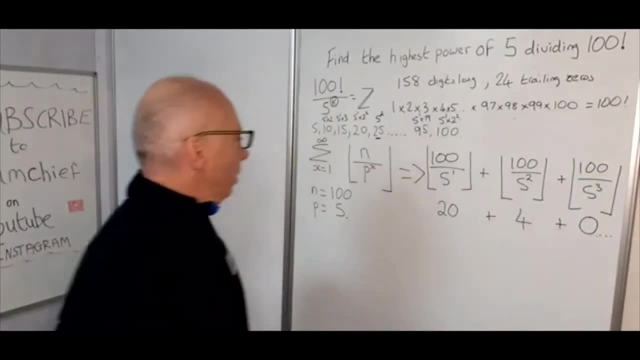 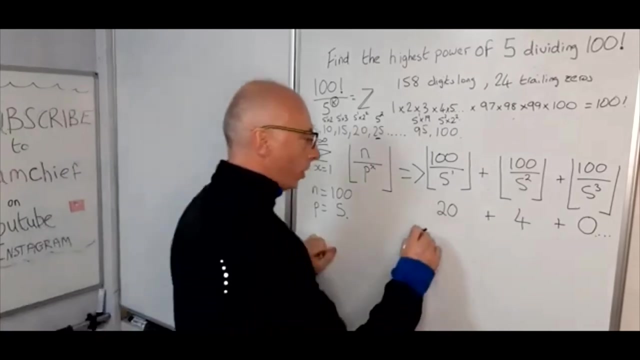 function, that will become zero. and then, obviously, if we go five to the power of four, that will keep going to zero and zero on forever and ever. so if we add up these numbers here, we have 20 plus 4, so that's going to give us 24.. 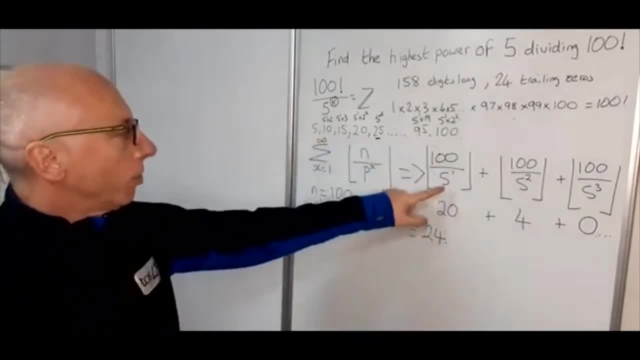 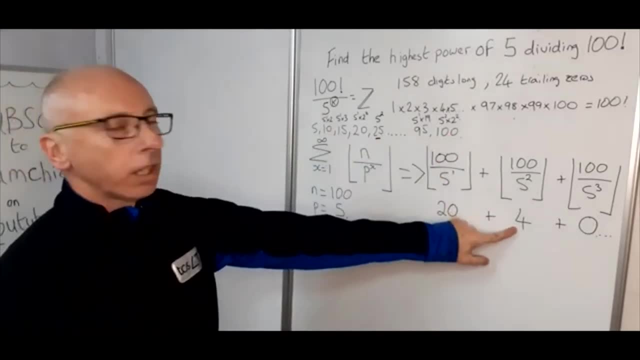 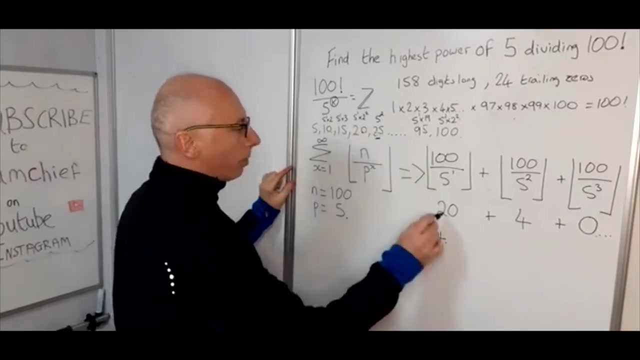 so if you work out along the line here all the way to 100, five to the power of one, there'll be five, 20 of those along the line, including four which are square numbers. so 5, 10, 15, 20, 25, going along the line, that'll be 20 digits, of which four will be square numbers. so we'll have 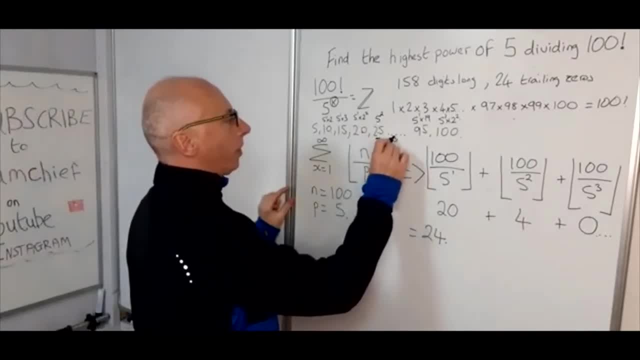 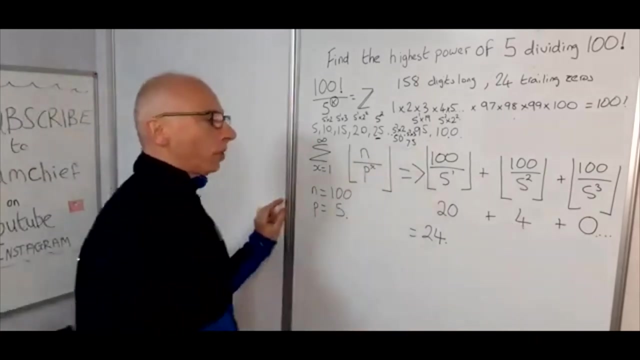 five squared, which is 25, we'll have 50, which is five squared times two. there'll be a seven, 25, which is five squared times three. then, of course, here we've got the 100, which is five squared times two squared. so that shows us where the fourth comes from, and the 20 will be all the.